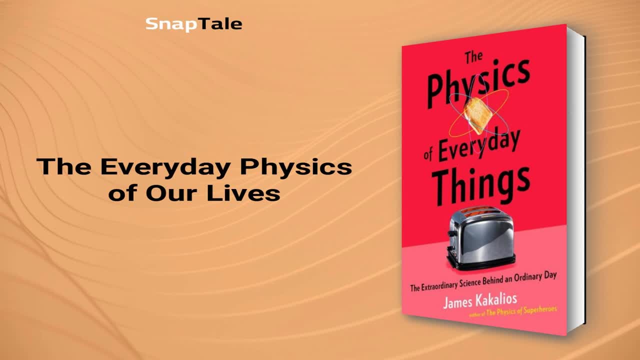 Have you ever stopped to think about how the gadgets and devices we use every day work In The Physics of Everyday Things? author James Kekalios breaks down complex concepts from the world of physics into easily digestible nuggets of knowledge. He draws our attention to the 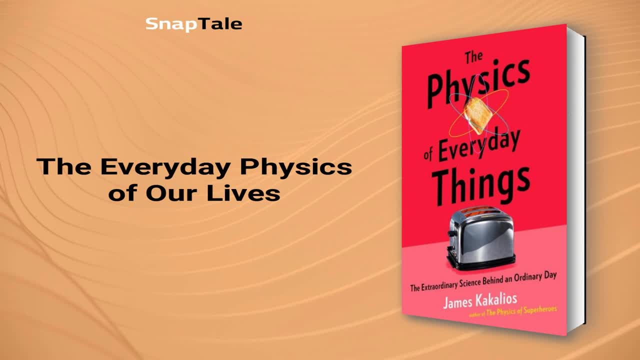 fascinating ways in which physics shapes our daily routine. Kekalios begins with the electromagnetic waves that power our alarms and coffee makers, explaining how the principle of conservation of energy governs all aspects of our lives. James Kekalios, author of The Physics of Superheroes. 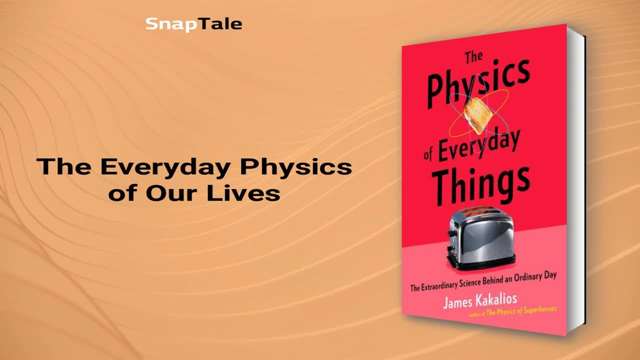 explains the mechanics of batteries and transformers, detailing how they power our toothbrushes and other devices. When it comes to transportation, Kekalios is just as enlightening. He walks us through the inner workings of the internal combustion engine and explains how our GPS systems connect to 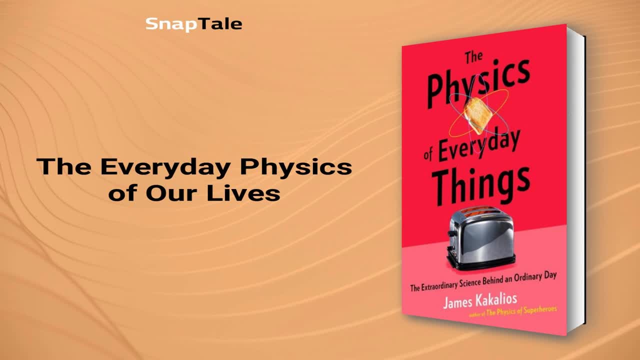 satellites in space. We learn how our E-ZPass devices communicate with tollbooth receivers and how our wireless devices connect to routers via radio waves. Kekalios also explores the world of touchscreens, revealing the ingenious design behind these ubiquitous interfaces. He explains the difference between resistive and capacitive touchscreens, and 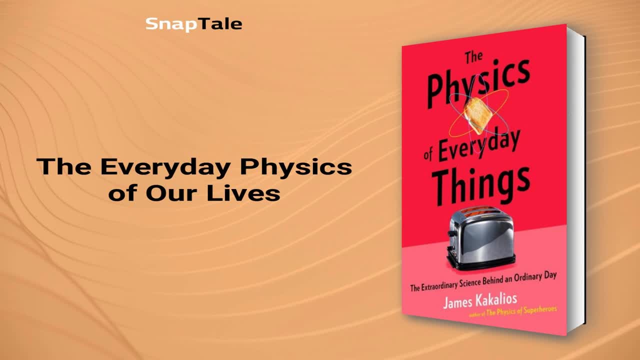 why the latter won't work if we wear gloves. Throughout the book. Kekalios peppers his explanations with interesting tidbits about the science behind our favorite gadgets. We learn, for example, that airport body scanners use microwaves that are weaker than those in a 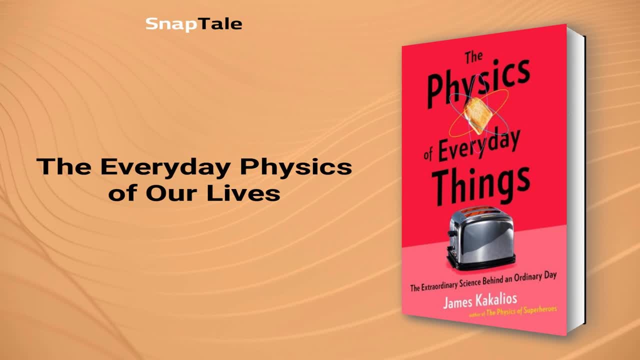 microwave oven. We also discover how photodiodes in our cameras use light to create precise images that match colors based on the wavelength of that light. Kekalios has a gift for making complex information accessible and engaging, for readers of all ages and The Physics of Everyday Things. 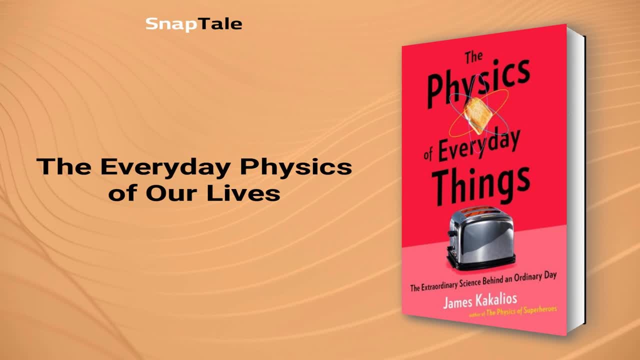 is no exception. By the end of the book, you'll have a new appreciation for the physics that makes modern life possible. Physics Made Accessible. Kekalios' Passion for Physics is the most important thing in the world of technology. Physics is evident in his book, which assumes an understanding of scientific concepts and vernacular. 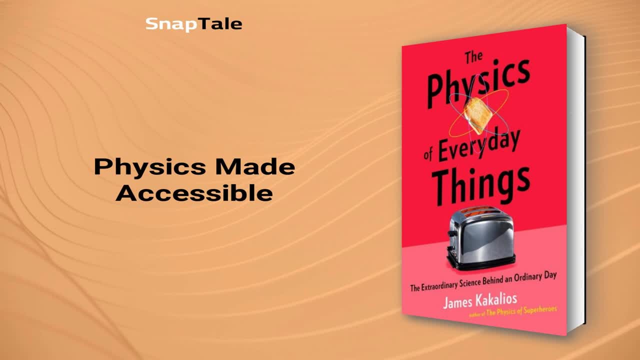 Though his day-to-day narration can be tiresome, the book is a good starting point for science enthusiasts. With his folksy approach, Kekalios appeals to curious young readers inclined toward science who are interested in learning how physics can manifest in their daily lives.